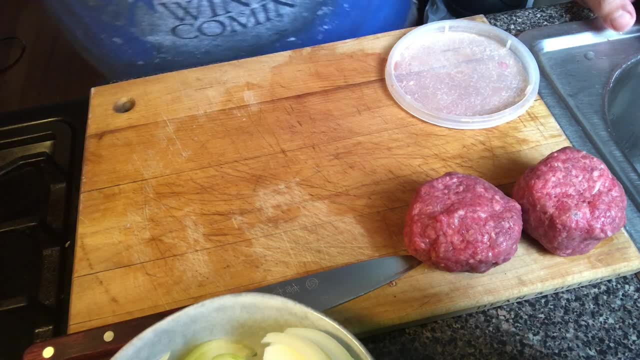 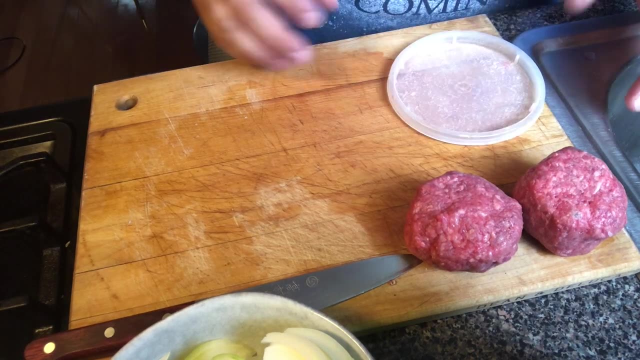 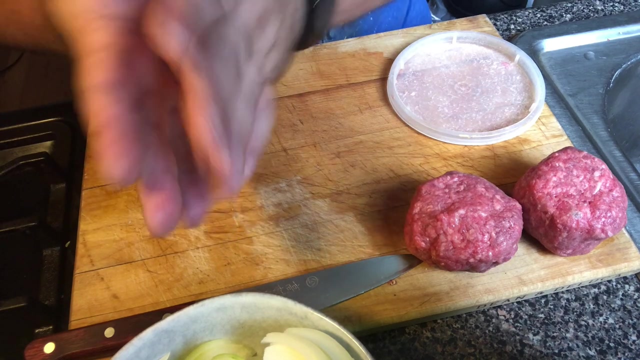 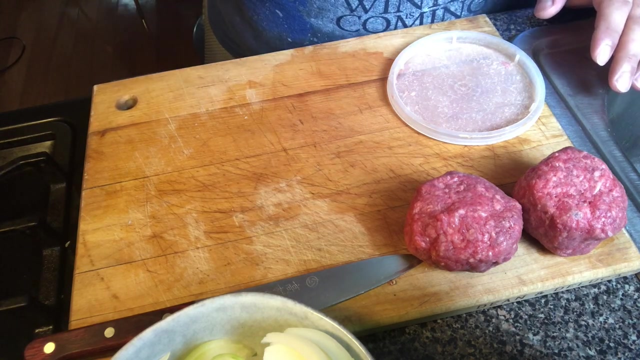 What's up guys? Chef Dave here with another quick tip. I was in the middle of a burger video and I thought to myself: you know what? I should show everybody how to make round burgers kind of easy. I know a lot of times you're sitting there forming and forming and padding and padding and padding, which is fine, don't get me wrong. But if you're the kind of person that kind of really wants sort of evenness, this is a good little way to do it. So this really works with four ounce burgers. 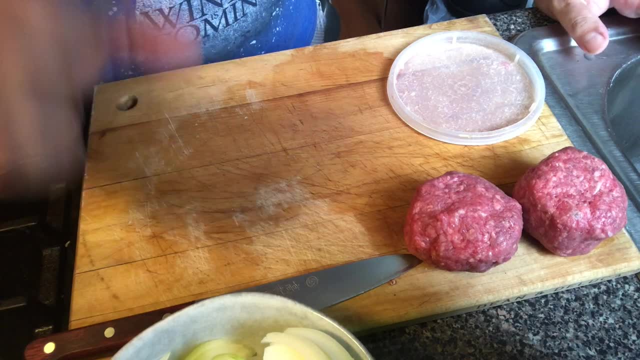 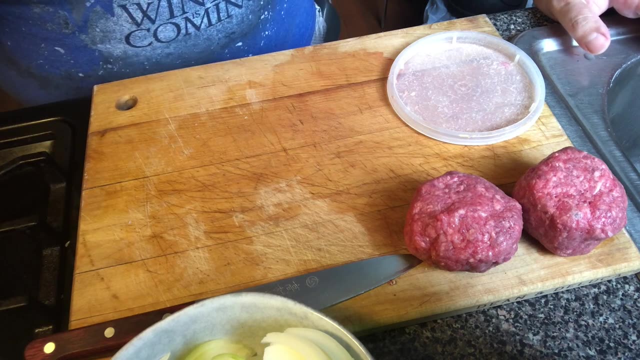 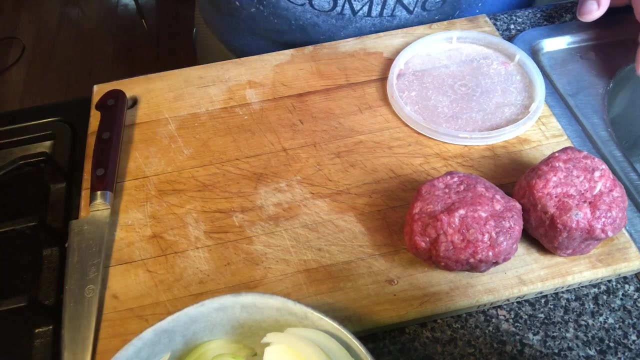 Which is actually, if I'm not doing like a steak burger or a thick mamma jamma, then I always only do four ounce burgers, especially for like griddle burgers or saute burgers, things like that. So this is a neat little trick that was actually taught to me by a friend of mine, Rich Parenti. 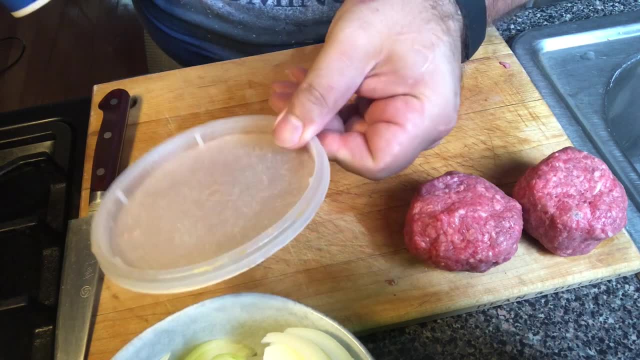 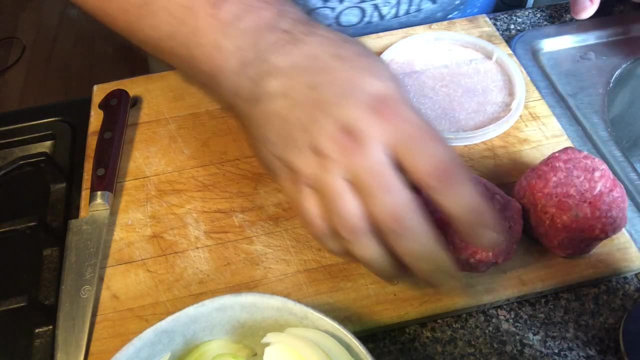 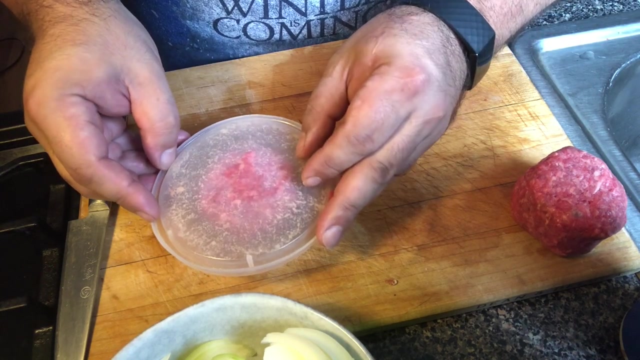 All you need is Chinese food, Chinese food, wood, something round. I'm just using my salt, something on the flat bottom, And all you do is: I've pre-portioned four ounces of ground beef And what you do is you flip it over, flip your lid, give it a nice little press. 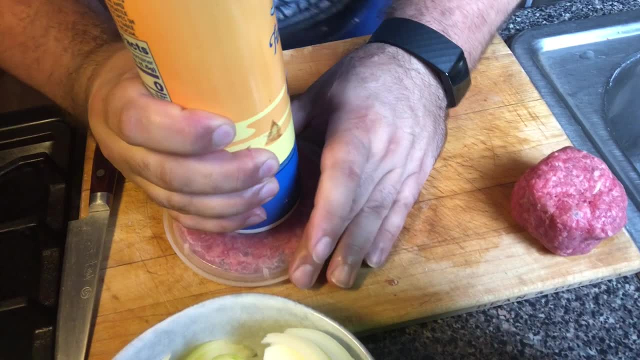 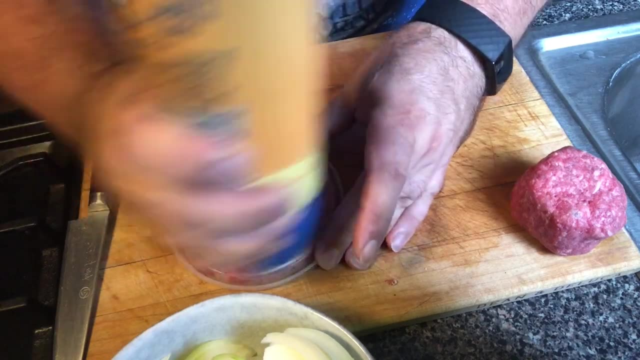 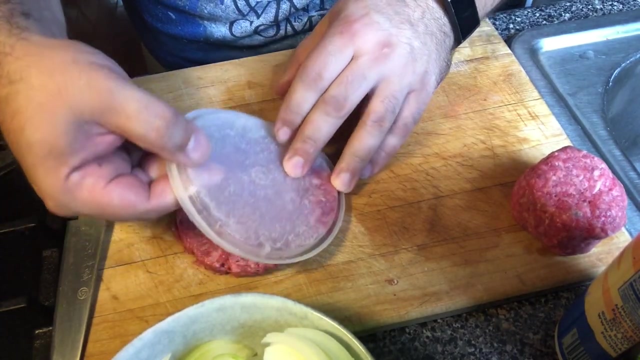 When you get there, when you get to here, you take your guy here, your salt container or whatever, give it another little press and just push it Boop, boop, boop And take it off, and then you have. 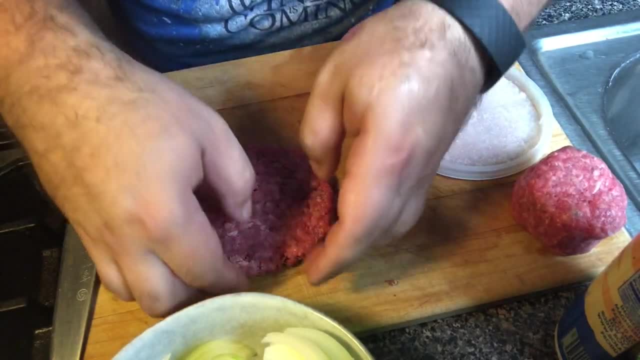 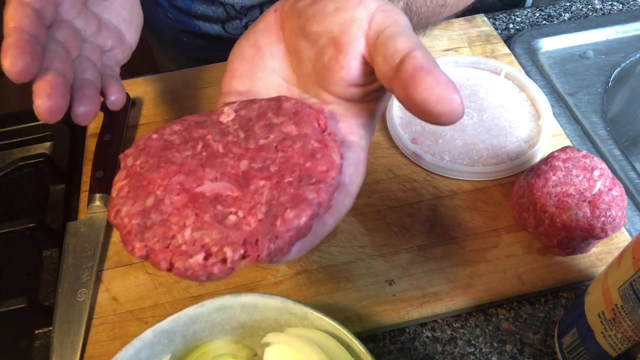